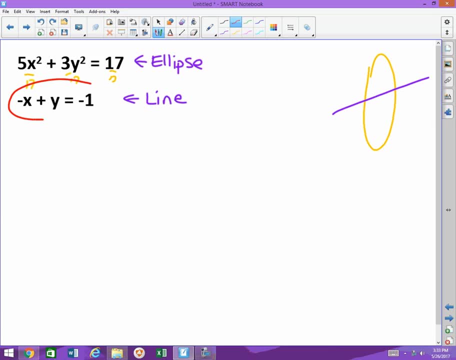 take one of the equations to solve for one of the variables. I think I will take that equation and solve for y by adding x, And so y equals x minus 1.. And then we can substitute this into the top equation for y, So we would have 5x squared plus 3 times x minus 1 squared equals 17.. And now we have to get it in the proper form and square some things and get everything to solve it. 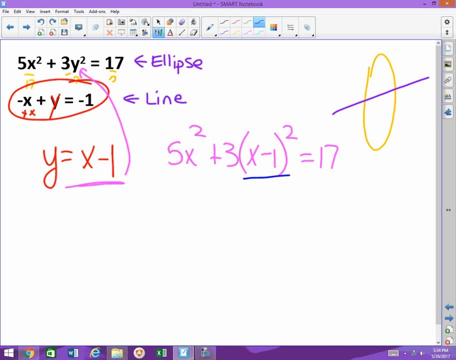 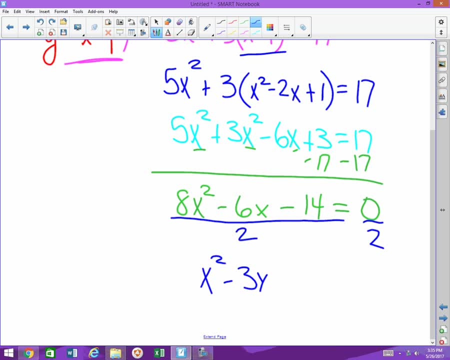 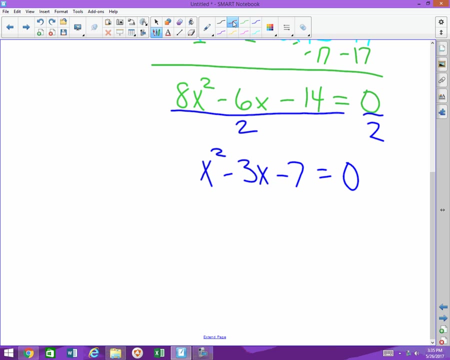 And that will get me: x squared minus 3x minus 7 equals 0.. And are there factors of a negative 7 that gets you to a negative 3? No. So therefore, you are going to say x equals plus and minus. 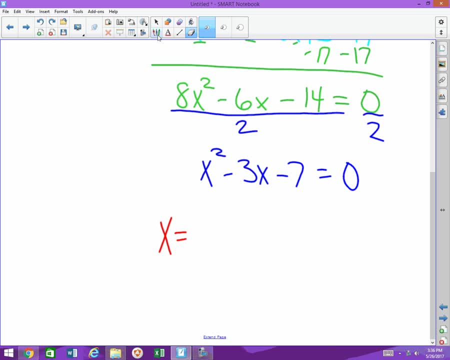 No, not plus and minus. It's 3 plus and minus. the square root of negative, 3 squared minus, 4 times 1 times negative, 7 all over 2 times 1.. That is 9 plus 28 is going to be 3 plus and minus. the square root of 37 all over 2.. 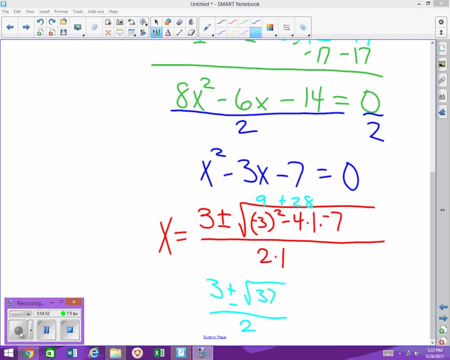 That's just a wow moment. again, I'm trying to go through this too quickly and I can't even do things properly And I'm sure you're all freaking out at that point because I made another mistake. So let's see, We've got to back up because when you divide here by 2,, 8 divided by 2 is 4.. 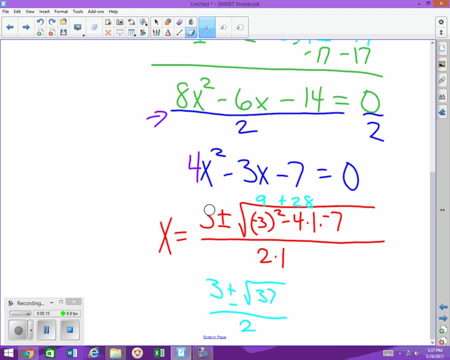 So that should be a 4 there. Now I think this might be factorable, And if not you can still use a quadratic formula. But let's say it is Hey. factors of 4 are 4x and x. 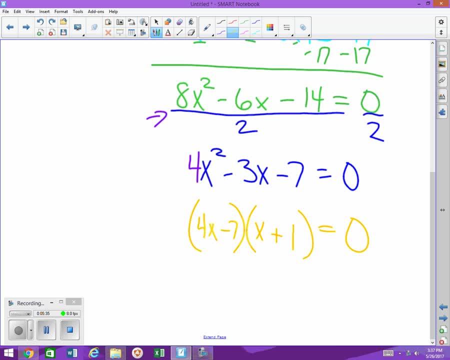 And if we put a negative 7 there and a plus 1 there, that's a negative 7x when you multiply those And a positive 4x, which makes a negative 3x, which is what we have to get to. 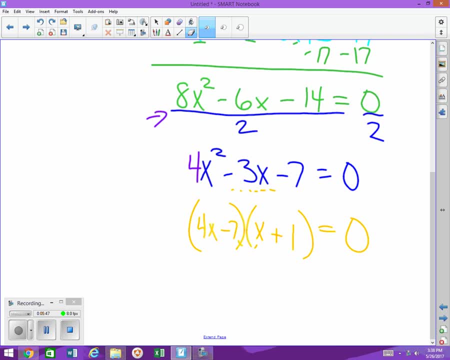 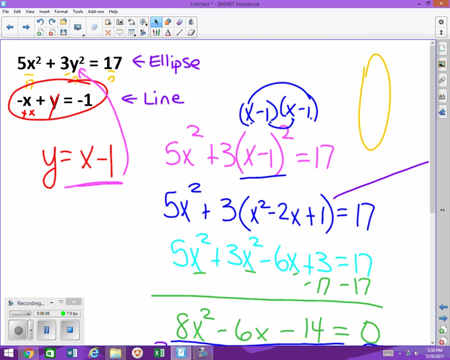 So therefore, it's factorable, And In this case x is equal to 7 fourths, And in that case x is equal to a negative 1.. Now, had you done this and gotten some imaginary solutions? well then, that means you're looking at a graph where that and that do not intersect. 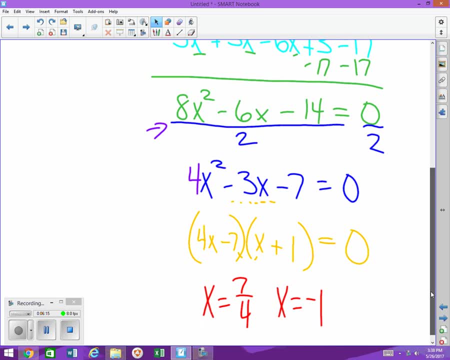 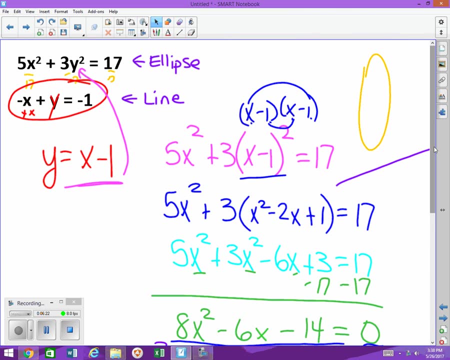 But we got two x values here, And so now we have to substitute those two things in, And we can use any one of the three that we have over here, which would be this one here, that one there or that one there. 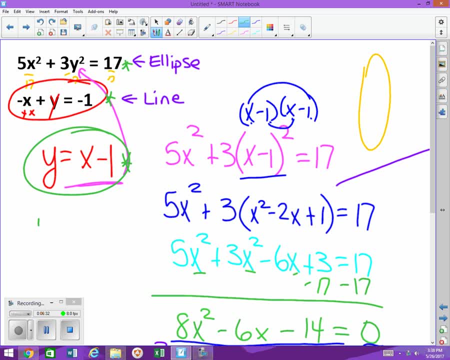 And I think this one would be the one-to-one you'd want to work with. So y equals 7 fourths minus 1.. And in that case, 7 fourths minus 1 is 3 fourths. So therefore, one of the equations: 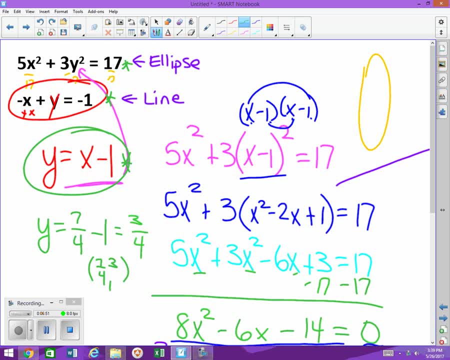 One of the equation coordinates is 7 fourths, comma 3 fourths, And our other x value was a negative 1.. So we would have y equals a negative 1 minus 1, which is negative 2.. And the other coordinate where they intersect is a negative 1, negative 2.. 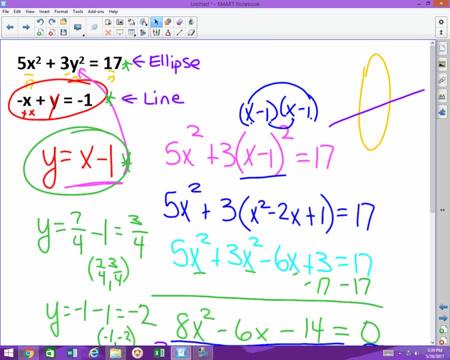 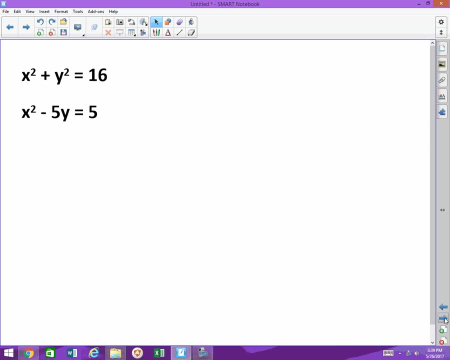 So we're looking at that type of a thing. Okay, There's one point, There's the other. Then our second equation: here We could use substitution on this one as well. Now, when you do substitution with something like this: pick a variable. 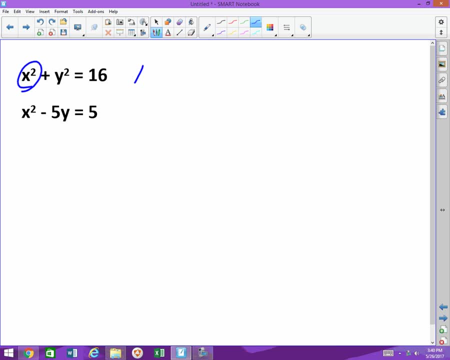 If you wanted to, you could solve this for x squared and get: x squared equals 16 minus y squared, And don't go down all the way to x, Just go to x squared. And now take that and substitute it in for x squared and then finish it. 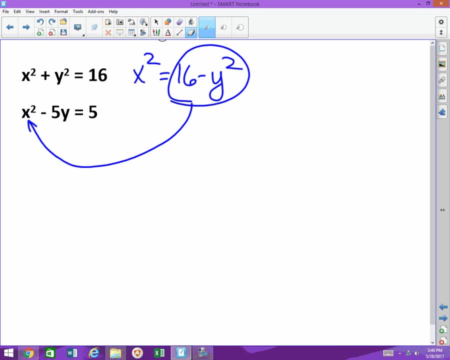 The other way is to use elimination. And so, in order to use elimination, Let's see, Let's eliminate the x squareds. Multiply this by a negative 1.. And you would get a negative. x squared plus 5y equals negative 5.. 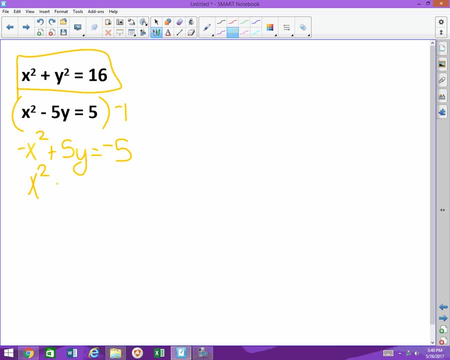 And then you're going to combine it with this one. So x squared plus y squared equals 16.. Now be careful, See if I can do this right, since I made a mistake on the last one. If you're going to add a negative x squared and a positive x squared, you get 0.. 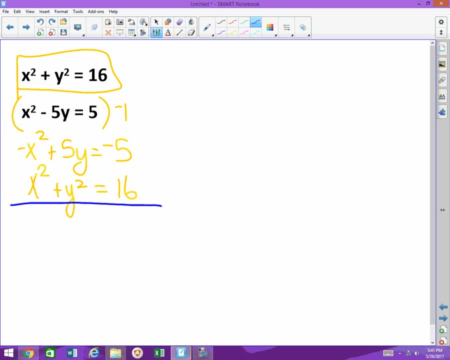 So those eliminate each other. Here you have a 5y, and there you have a y squared. Cannot add these together, So this turns into y squared, Y squared plus 5y, And then that equals 11.. And so now subtract 11.. 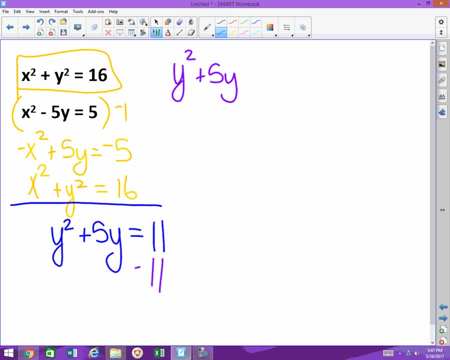 And you're going to have y squared plus 5y minus 11 equals 0.. And here we are going to need to use the quadratic formula. So to use the quadratic formula here you would have y equals a negative 5 plus and minus the square root of 5 squared minus 4 times 1 times a negative 11, all over 2 times 1.. 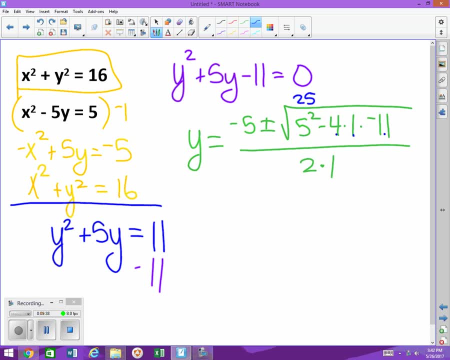 5 squared is 25.. 4 times 1 times 11 is 44. And it would be plus And 25 and 44 is 69. And so now we have a negative 5. Plus and minus the square root of 69, all over 2.. 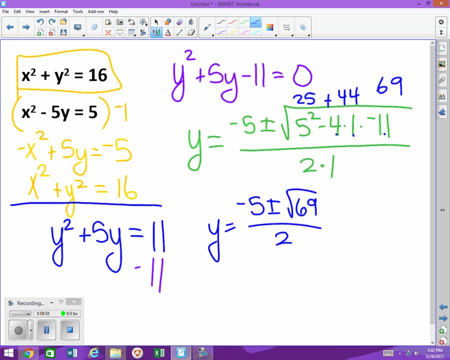 And that's what y equals. And now to get the decimal approximation of those, that would be 1.6533 repeating, So let's just say 1.65.. And a negative 6.65 repeating with the 3.. And so we'll just say a negative 6.65. 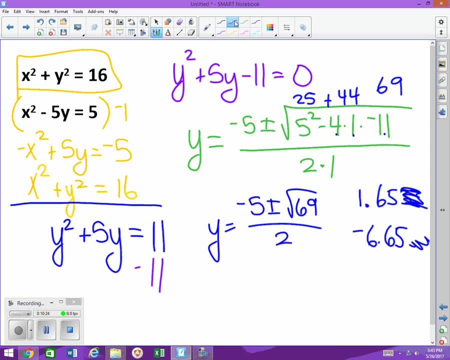 That's the two y values, And then we have to figure out the x values. Choose either one of the two equations. I am going to choose this one. So we have x squared minus 5y equals 5.. And so then you have to substitute 1.65 in for y. 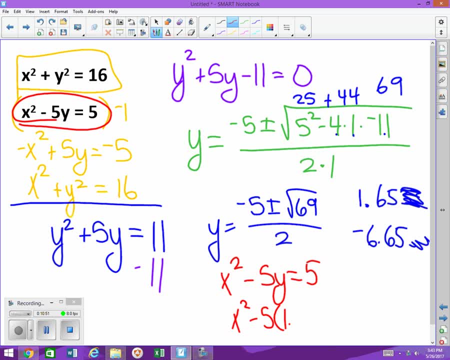 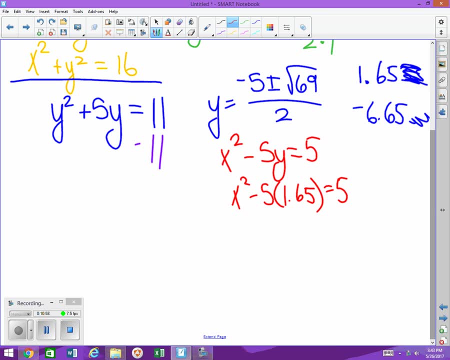 So x squared minus 5 times 1.65 equals 5.. And the other equation would be: x squared minus 5 times a negative 6.65 equals 5.. And let's see here: 5 times negative 6.65.. 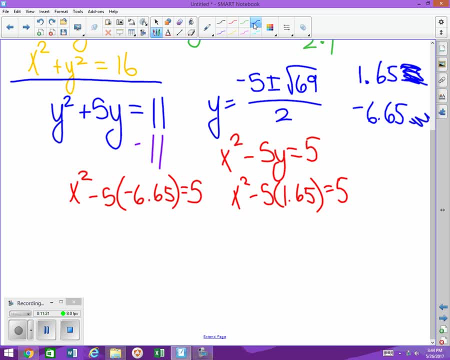 So that's going to be: x squared plus 33.25 equals 5.. So subtract that And you're going to get x squared equals some negative numbers. It's just going to be imaginary, So those aren't real. And here we have x squared. 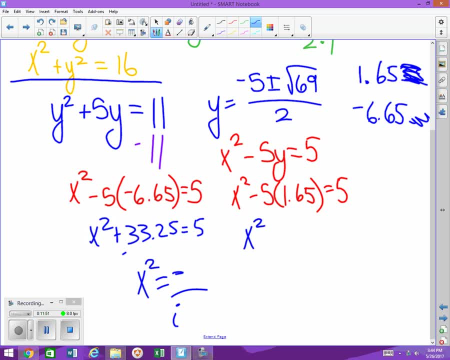 x squared minus 8.25 equals 5.. And then, when you add 8.25 to both sides, you have x squared equals 13.25.. And then, when you take the square root of x squared, you have x squared equals 13.25.. 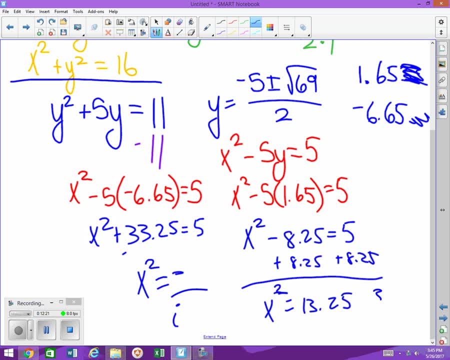 And then, when you take the square root of that, you're going to get 3.64.. And so you have 1.65 comma 3.64.. Don't forget, this is plus and minus, for x equals. And then you would also have 1.65 comma negative 3.64.. 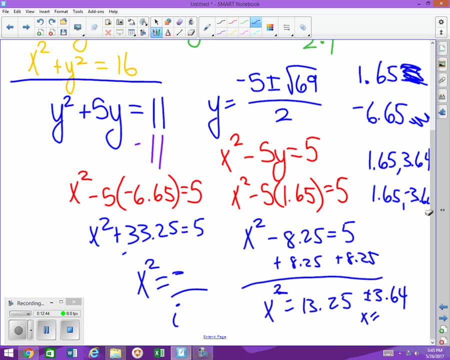 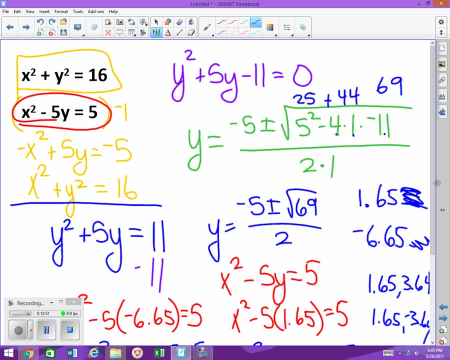 Whoops, Oops, and those would be your two coordinates. So what are we looking at here for graphs? Here we have a circle and here we have a parabola, And since they are intersecting in two places, maybe it's a parabola that goes like: let's see that. 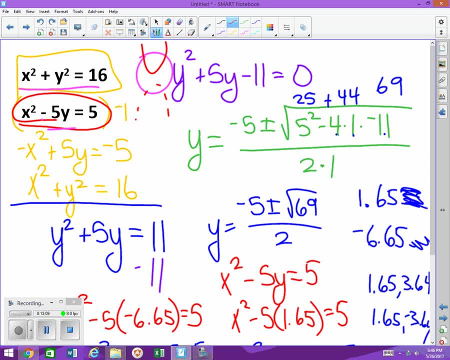 Or it's possibly a here, And so those are your two points. Now you also could have a circle and a parabola, say opening to the right, that does this, Or it's like that and there's no solution, Or maybe it comes and it just touches. 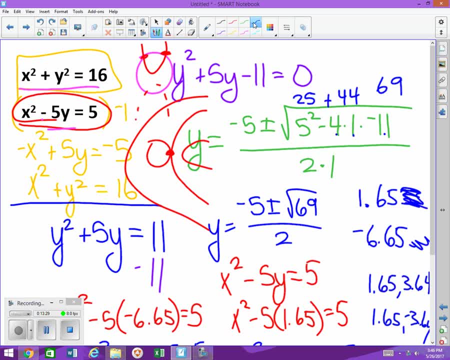 and there's only one solution. Or it could be a parabola that comes and does one of these things, where it goes through there and there's one solution and touches and then goes back And there's a second solution and a third one. 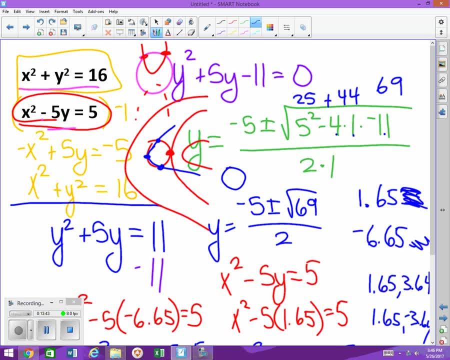 That could be happening. Or you could have a circle, and it could go like that, where you have four solutions. So it all depends on what you're looking at, And those are the different ways that you can use to solve equations and come up with the intersection points. 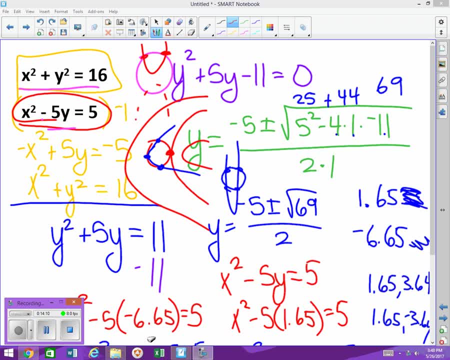 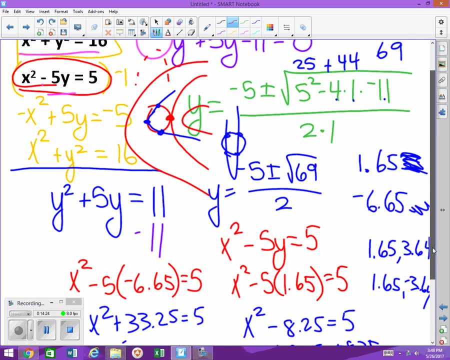 Hang on, We made another mistake, Sorry Here. when I solved these, you guys didn't do it, I did. We had our two x values Or no? these are our two y values first And we tried to substitute them in.